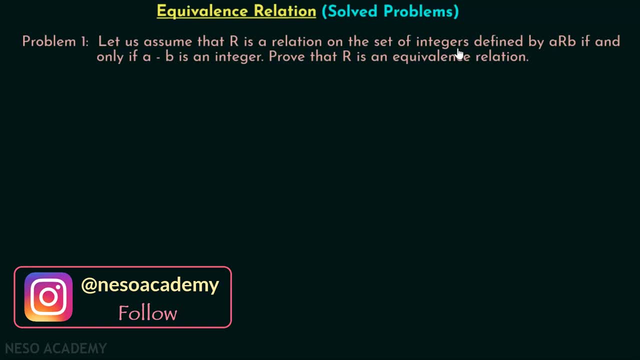 So we have a relation R which is defined on set of integers. And let me tell you that relation R is nothing but set of all ordered pairs of the form A, comma, B, if, and only if, A minus B is an integer. Okay, 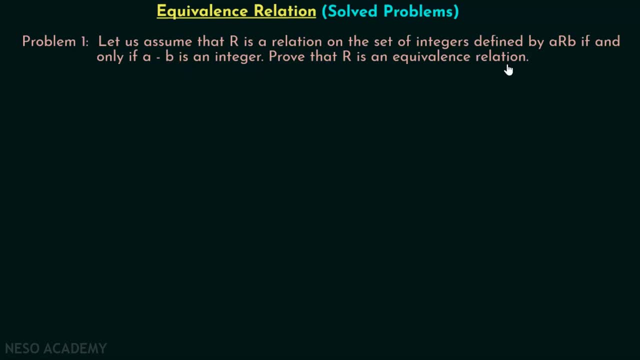 We have to prove that R is an equivalence relation. Okay, Let us assume that set A represents set of all integers. Here you can see: the set represents set of all integers. R is defined on set A and R is nothing but A related to B. 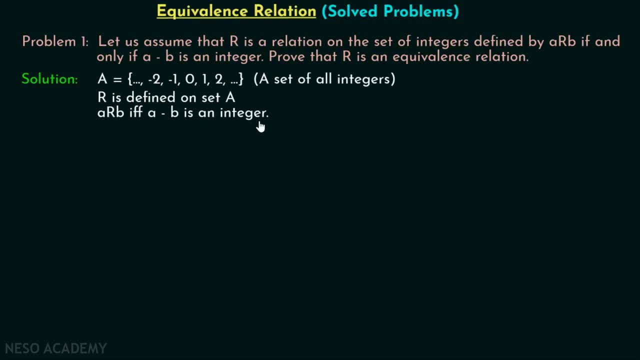 if, and only if, A minus B is an integer. This is, according to the question, right. We have to prove that this relation is an equivalence relation. For this, first we will check whether this relation is reflexive or not. We know the definition of reflexivity. 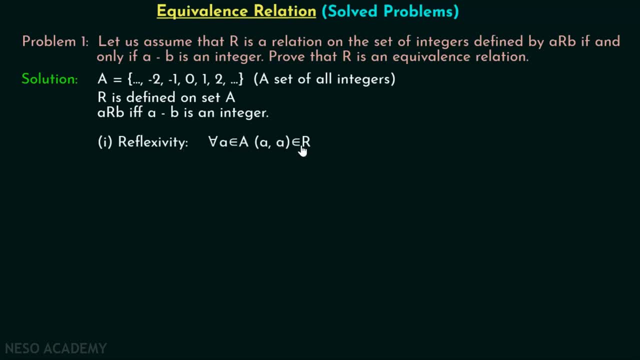 For all: A belong to A. A comma A must belong to R. right For every element: A belong to the set A. A comma A. this ordered pair must belong to this relation: R. Now what is the meaning of A comma A belong to R. 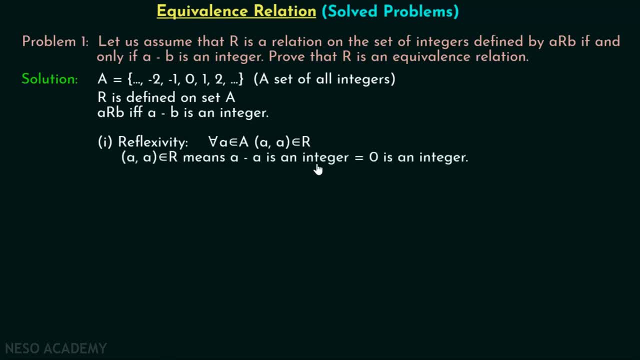 A comma A belong to R means A minus A must be an integer right, Because we know that A is related to B if, and only if, A minus B is an integer. Or in other words, we can say that A comma B belong to R. 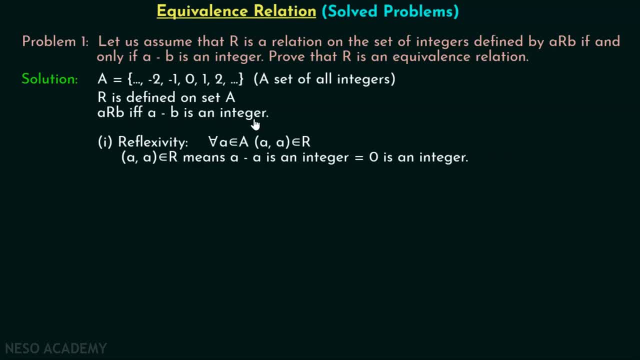 if, and only if, A minus B is an integer. Here we are saying that A comma A belongs to R. This means that A minus A must be an integer. What is A minus A? A minus A gives zero right. Zero is an integer. 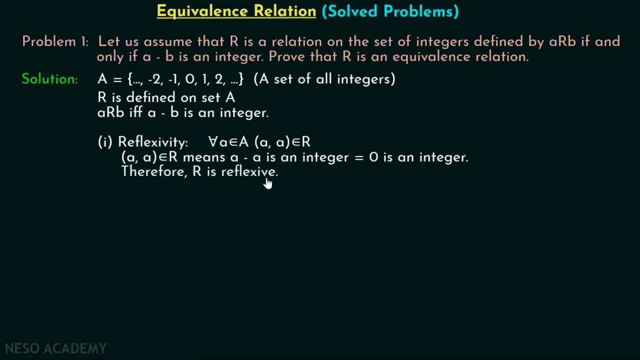 We know that zero is an integer right. Therefore, R is reflexive, Isn't that? so This is very simple right. This relation is reflexive. Now let's just identify whether this relation is symmetric or not. We know the definition of symmetry. 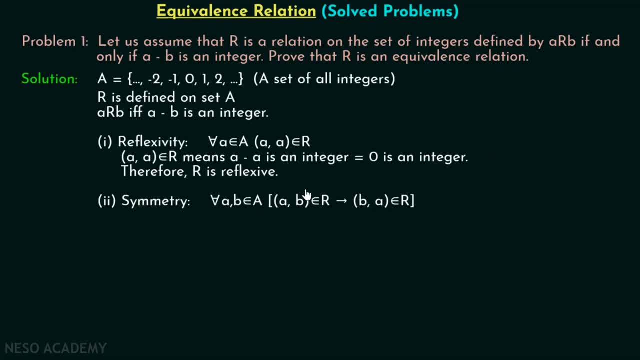 For all A comma B belong to set A A comma B. this ordered pair belong to R implies B comma A belong to R, right. What is the meaning of A comma B belongs to R? A comma B belongs to R means A minus B is an integer. 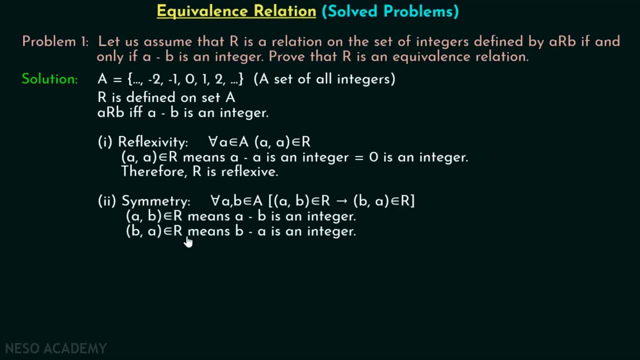 What is the meaning of B comma A belongs to R. B comma A belongs to R means B minus A is an integer, is an integer. Simple Now, according to this definition, it is given that a minus b is an integer. Let's say a minus b is an integer. Fine, If a minus b is an integer, then b minus a which? 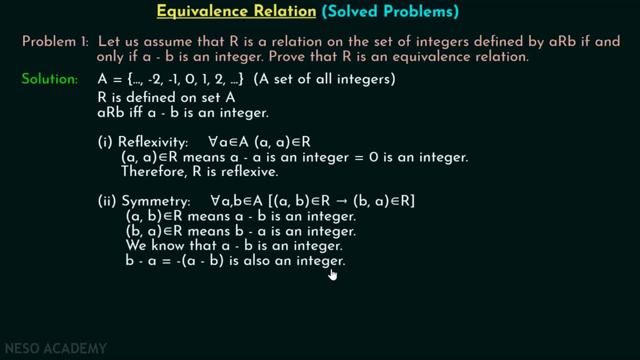 is nothing but minus a minus b is also an integer. We can write b minus a as minus a minus b. This is also an integer right. Therefore relation R is symmetric. From this. we have to prove this. A minus b is an integer. We have to prove that b minus a is also an integer. Here we have proved. 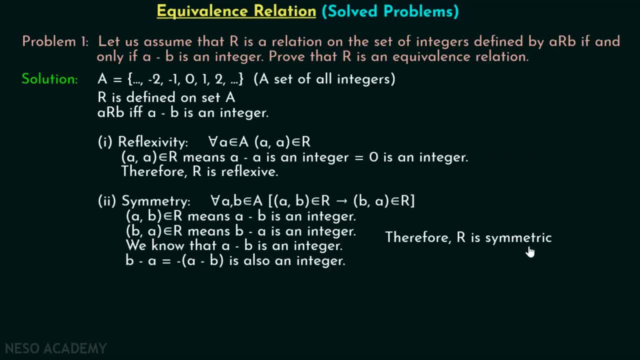 that b minus a is also an integer. Therefore, R is symmetric, Simple. Now let's see whether this relation R is transitive or not. According to the definition of transitivity, for all, a comma b comma c belong to set A. a comma b belong to R and b comma c belong to R implies a comma c belong. 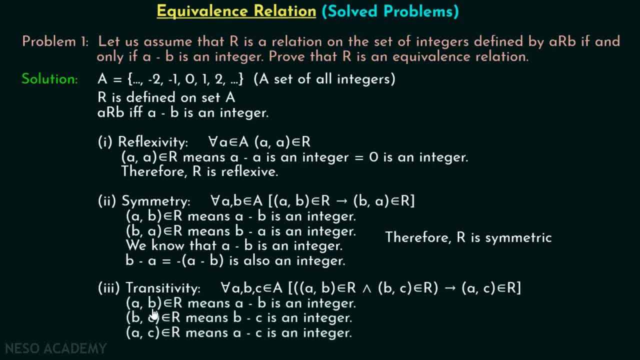 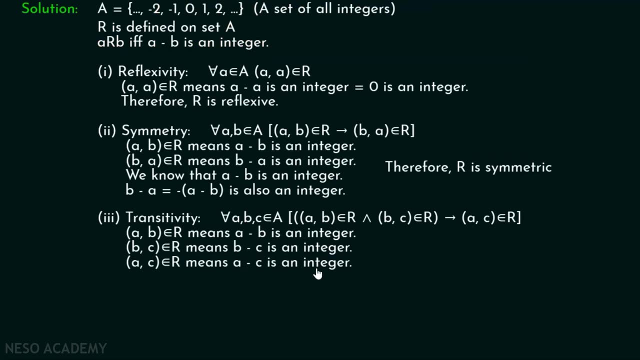 to R. What is the meaning of a comma b belongs to R. This means a minus b is an integer. B comma c belongs to R means b minus c is an integer. A comma c belongs to R means a minus c is an integer. right From these two. we have to prove that a minus c is. 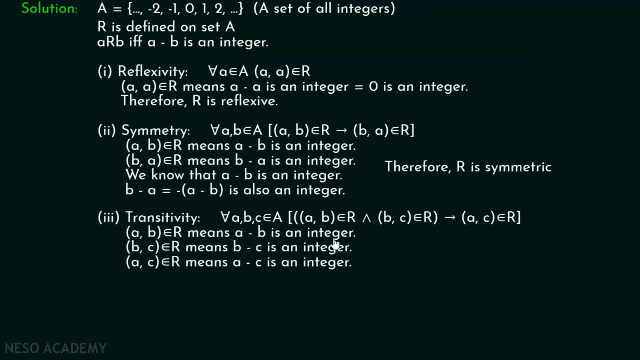 also an integer. That is, if a minus b is an integer and b minus c is an integer, then a minus c must also be an integer. Let's take the addition of these two: a minus b plus, b minus c. We know. 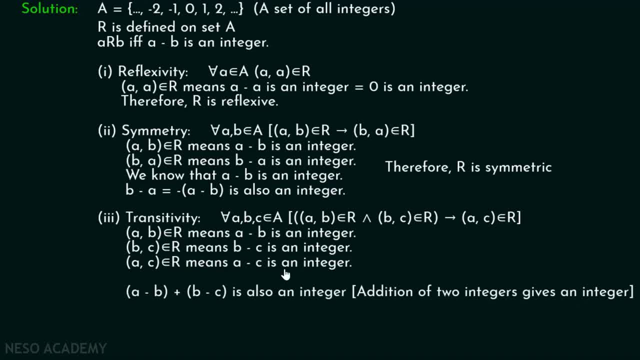 that a minus c is an integer, because addition of two integers gives an integer right. A minus b plus b minus c is actually equal to a minus c, As we know that a minus b plus b minus c is an integer. therefore a minus c is also an integer. Therefore, R is transitive, Isn't that? so We know? 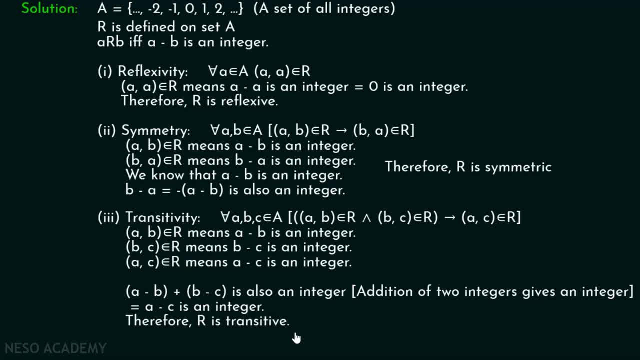 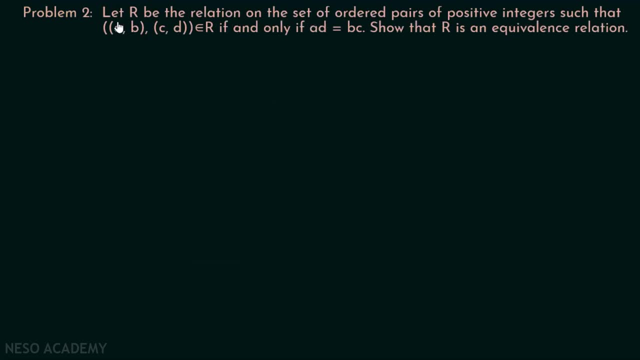 that relation. R is reflexive, symmetric and transitive. Therefore, R is an equivalence relation. There is no doubt about this. right Now let's see problem two. So let R be the relation on the set of ordered pairs of positive integers, such that this ordered pair 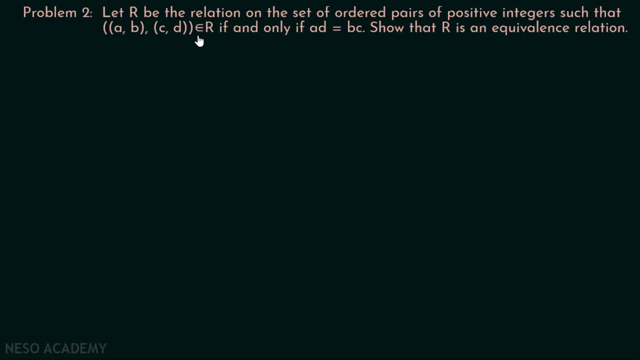 where first element and second element are ordered pairs belong to R if, and only if, ad equal to bc. Show that R is an equivalence relation. We have to show this relation is an equivalence relation. right? Let us suppose that a is the set of ordered pairs of positive integers. okay, That is. 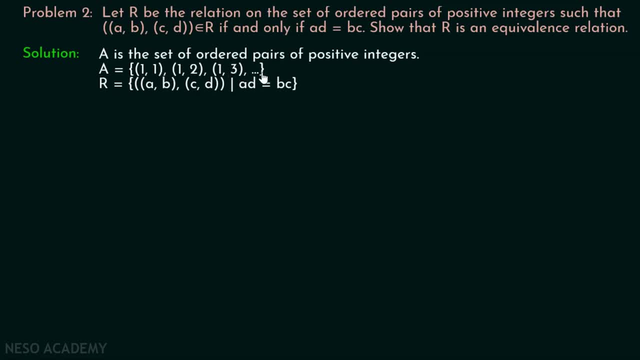 a is nothing but set of all ordered pairs of positive integers, Because we know that R is defined on the set of ordered pairs of positive integers. right, R is defined on this set, which is nothing but set of all ordered pairs of this form, where ad is equal. 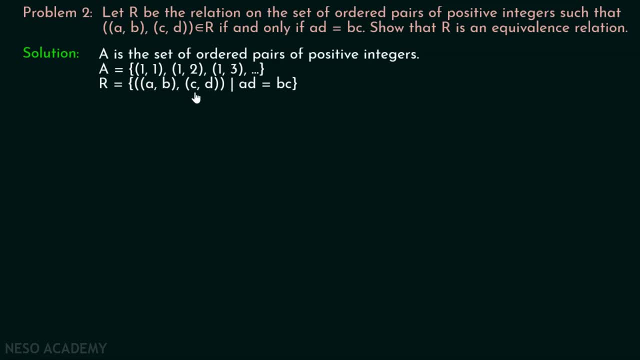 to bc, a into d is equal to b into c. fine, Here you can see that the first element of this ordered pair is itself an ordered pair, and second element is also an ordered pair. okay, So this is our relation. We have to show that this relation is an equivalence relation. So let's say that a is the. 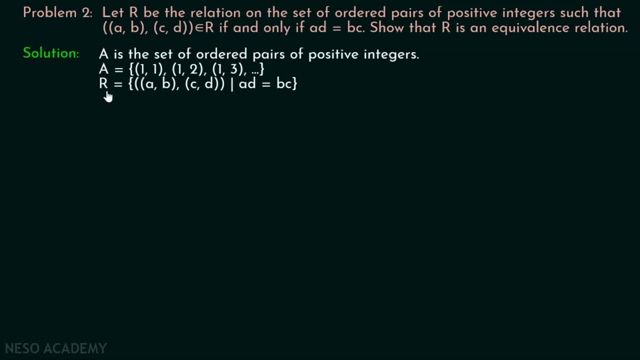 set of all ordered pairs of positive integers, right. So we have to show that this relation is an equivalence relation. For this, we have to show that this relation must be reflexive, symmetric and transitive. First, we will show that this relation is reflexive. We know the original definition of. 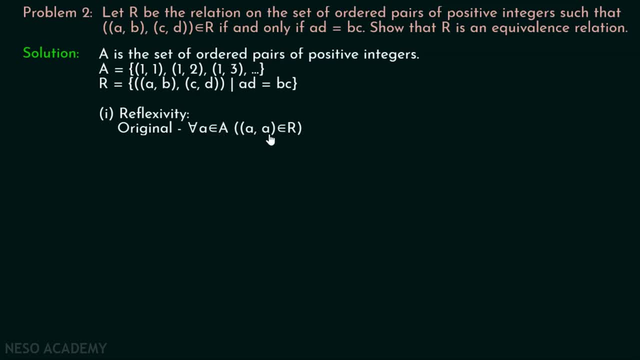 reflexivity For all. a belong to a, a comma a must belong to R. Here, instead of a, we have an ordered pair because every element of set a is an ordered pair, right? So here we can replace this a by an ordered pair. So we have to show that this relation is an equivalence relation. For this we 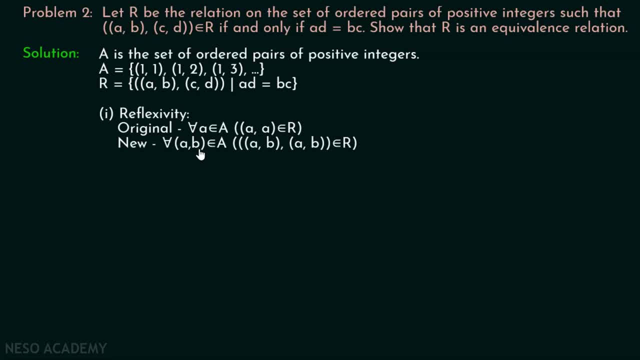 have to show that this relation is an ordered pair of this form: a comma b. It doesn't matter whether you choose c comma d, e comma f or any other letter combination. Here I am mentioning these two letters, a and b. Here I have written for all: a comma b belong to a that is set a. 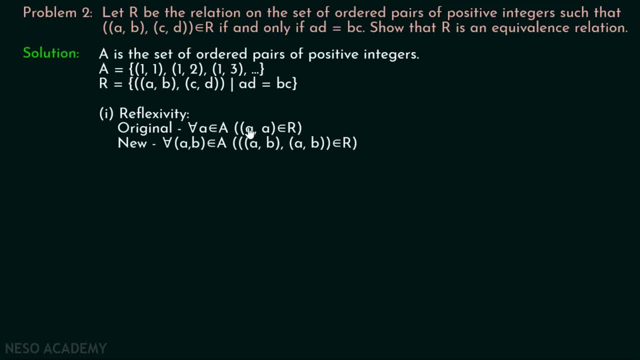 a comma b. comma a comma b belong to R. Just replace a by a comma b. That's it. This ordered pair must belong to R. This is according to the definition of reflexivity. okay, This is our new definition. fine, This ordered pair belongs to R. Now, what is the meaning of this? 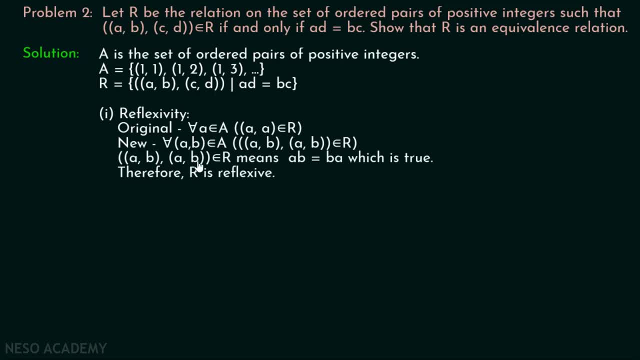 ordered pair belongs to R. a comma b, comma a comma b belongs to R means ab is equal to ba. This is, according to the definition, right. When this ordered pair belongs to R, then ad must be equal to bc. ad must be equal to bc Here. if this ordered pair belongs to R, then this: 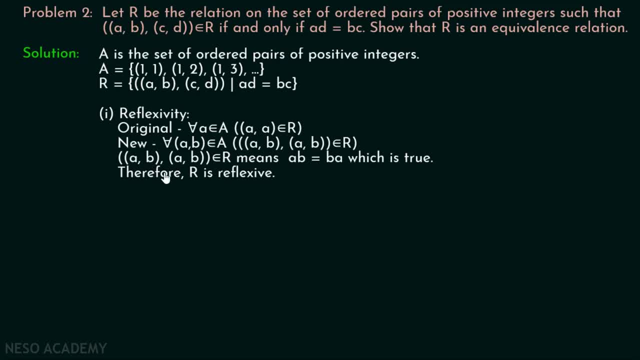 means a b must be equal to b a right. Is a b equal to b a? Obviously, this is true, right. Therefore, r is reflexive. As simple as that. Now let's see whether this relation is symmetric or not. 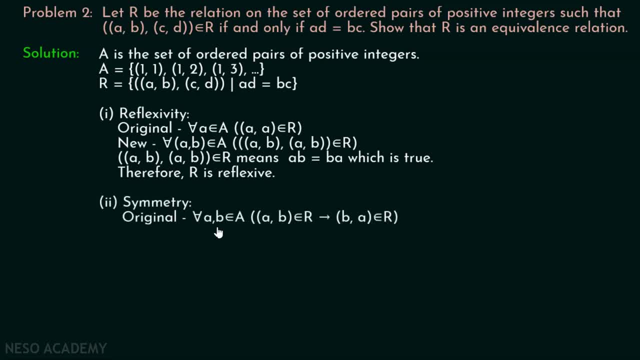 For this we must see the original definition of symmetry. For all a, b belong to a. a b belong to r implies b a belong to r. right Now the new definition looks like this: For all a, b, c, d belong to a. 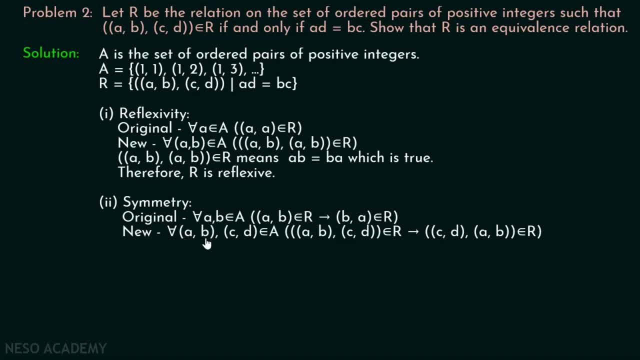 Here a is replaced by this ordered pair: a, b- Okay, some arbitrary ordered pair. And b is replaced by c, d, A different ordered pair. right For all. a, b, c, d belong to a, a, b, c, d belong to r implies c: d, a, b belong to r. 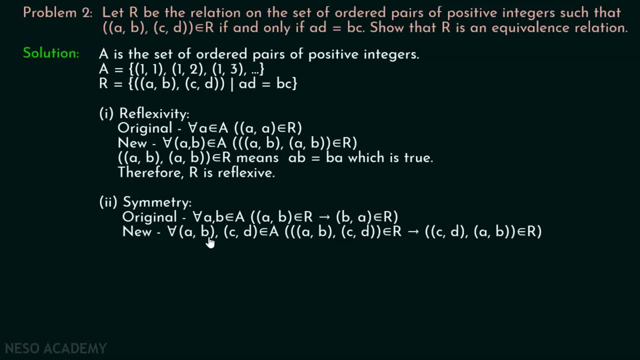 This is not very difficult to understand. Just replace a by a, b and b by c, d in this definition. Now let's see what happens. You will get this new definition right. What is the meaning of a, b, c, d? belongs to r. 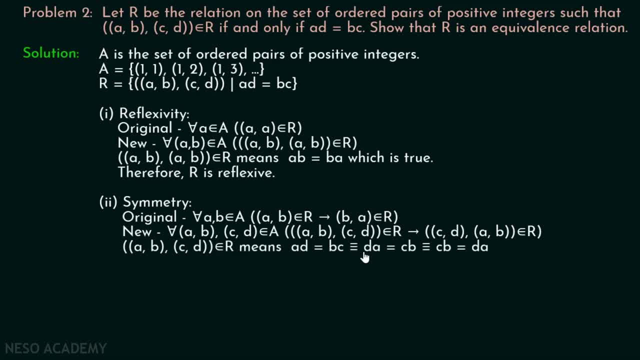 This means a d is equal to b c. And let me tell you: this is equivalent to d a equal to c b, And this is equivalent to c b equal to d a. right, There is no doubt about this. 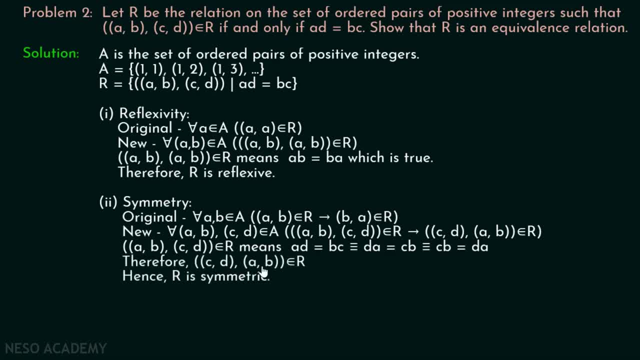 What is the meaning of c, b equal to d, a, c, d, a, b belongs to r, Isn't that so? This means, when a, b, c, d belongs to r, then c, d, a, b belongs to r. 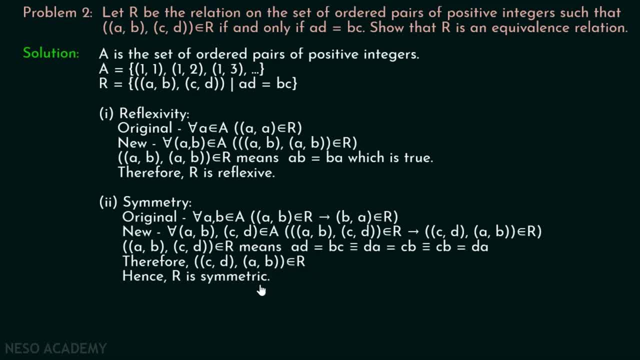 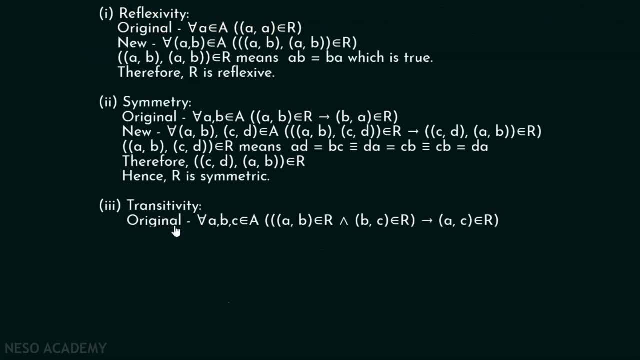 Hence we can say that r is symmetric, Isn't that? so Now let's see whether r is transitive or not. We know the original definition of transitivity For all: a, b, c belong to a, a, b belong to r and b- c belong to r. 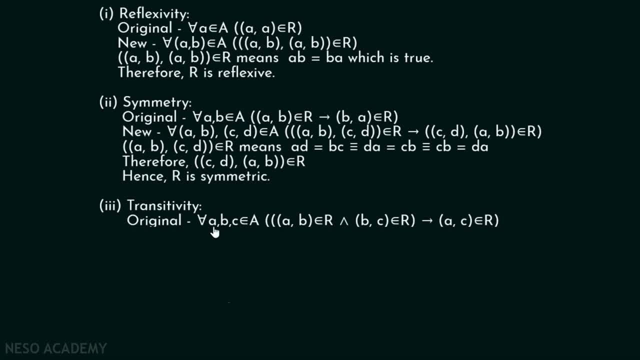 implies: a, c belong to r. Now here we can replace a by a, b, b by c, d and c by e, f. Okay, These three ordered pairs are different. Right For all. a, b, c, d, e, f belong to set A. 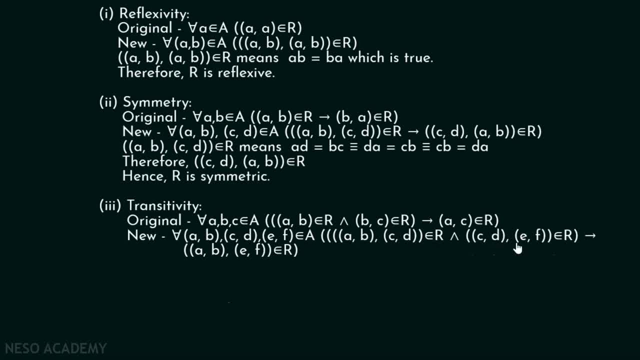 a, b, c, d belong to r and c, d, e, f belong to r implies a, b, e, f belong to r. Just replace a by a, b, b by c, d and c by e f in this definition. 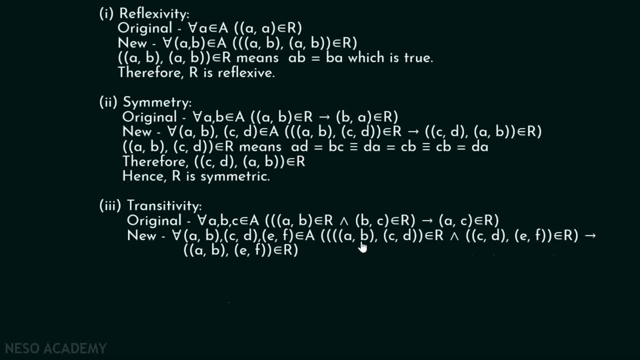 You will get this new definition Right. What is the meaning of a, b, c, d belongs to r? This means a, d is equal to b, c. What is the meaning of c, d, e, f belongs to r. 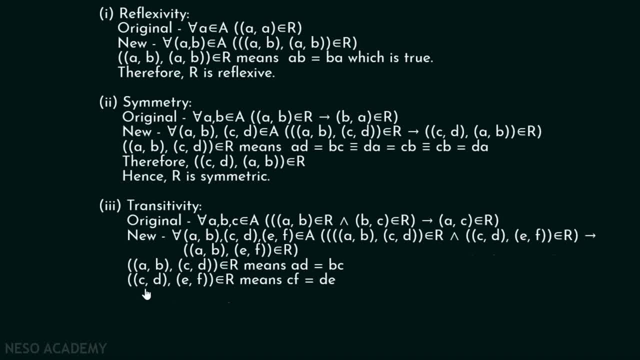 This means c f is equal to d e, c f equal to d e. Right, Let's say: this is one and this is two. Okay, From one it is clear that a is equal to b, c by d. 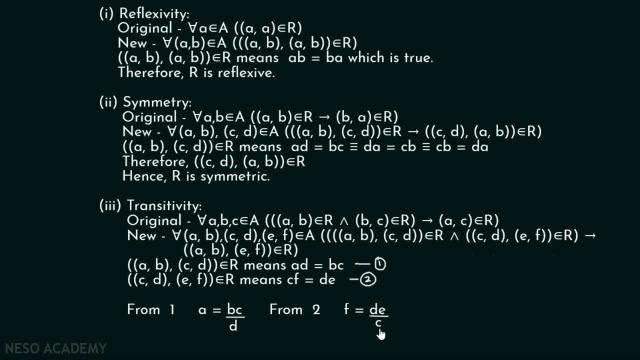 and from two f is equal to d e by c. Right, We can write this: Let's say this is three And this is four. Now, if we multiply three and four, then we will get a f equal to b, c by d into d, e by c. 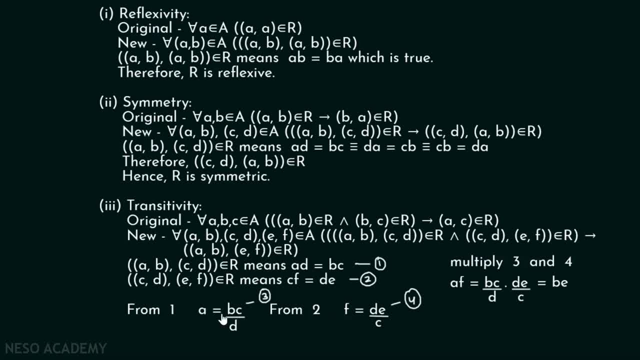 Right. a into f is equal to b, c by d into d, e by c. Right Now, if we see over here we can cancel c by c and d by d, We will get b? e Right. So a f is equal to b? e. 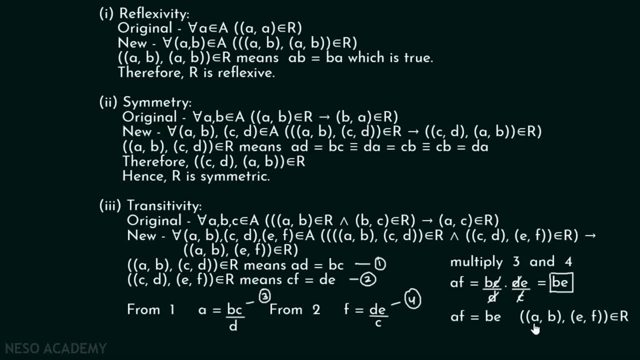 Now, what is the meaning of a f equal to b e? This is nothing but an ordered pair of this form: a, b e, f. This means, when a f is equal to b e, then this ordered pair belongs to r. 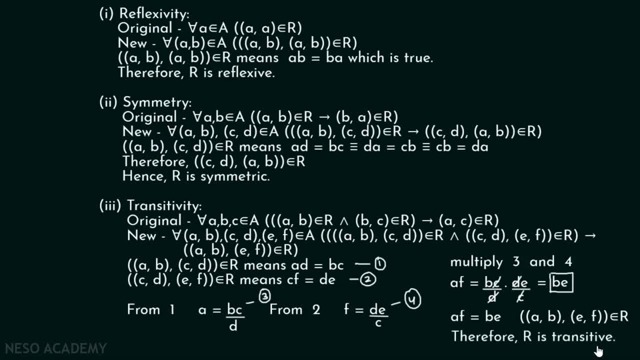 Right? Therefore, r is transitive, Isn't that so Relation r is transitive. Hence, it is clear that r is an equivalence relation, Because r is reflexive, symmetric and transitive, Right? Okay, friends, this is it for now.